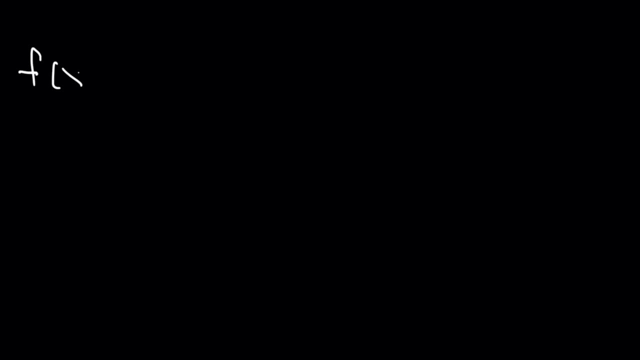 Consider the piecewise function f of x, and let's say that it's equal to 5x plus 3 when x is less than 2, and it's equal to 2x squared plus 5 when x is between 2 and 4, and then it equals x cubed minus 5x plus 3 when x is equal to 2x squared. 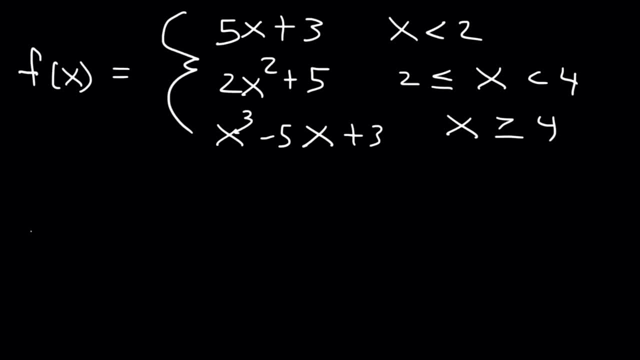 So what is the limit as x approaches 2 from the left side of f of x? So which portion of the piecewise function should we use Now as we approach 2 from the left side? should we choose a value like 1.99 or 2.01?? 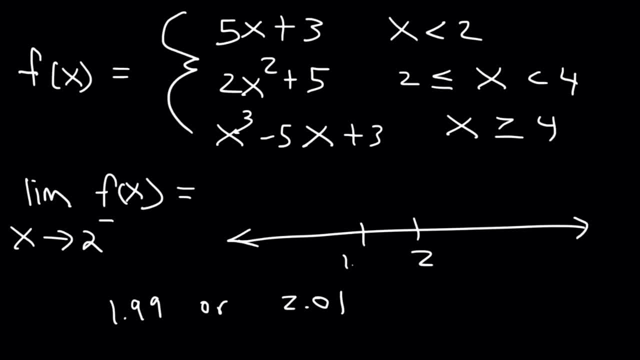 On a number line: here's 2., Here's 1.99 and here's 2.01.. So, as we approach 2 from the left side, should we choose a value like 1.99 or 2.01?? 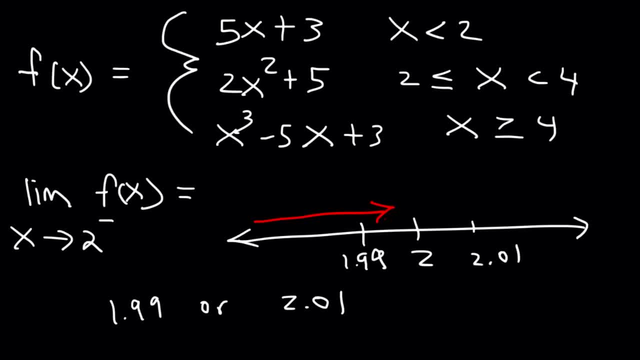 So, as we approach 2 from the left side, we have to pick a value that's less than 2, ideally 1.99.. So therefore, we need to use 5x plus 3, because that's when x is less than 2.. 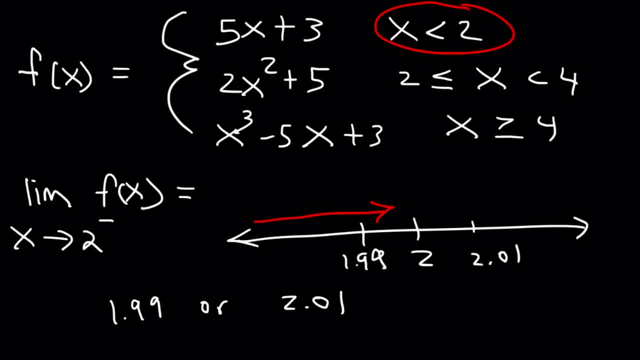 That's the left side of x, equals 2.. So it's going to be 5 times 2.. 2 plus 3, which is 10 plus 3, so that's equal to 13.. Now what is the limit? as x approaches 2 from the right of f of x. 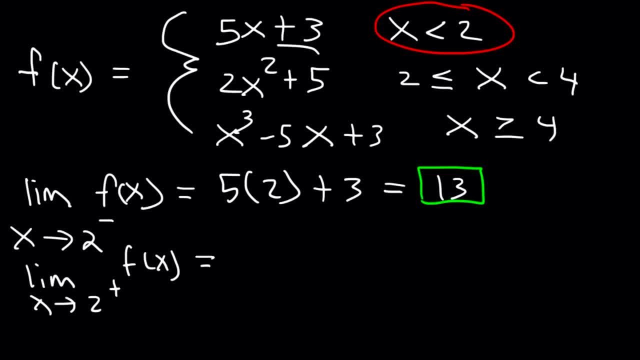 On the right side that is greater than 2, we need to use this portion of the piecewise function, 2x squared plus 5.. So it's 2 times 2 squared plus 5.. 2 squared is 4.. 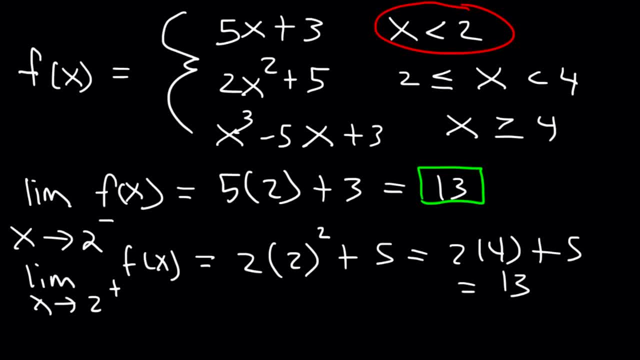 2 times 4 is 8.. 8 plus 5.. 8 plus 5 is 13.. Now let's find the limit as x approaches 2 from either side. So because these two are the same, you know that it's going to be 13.. 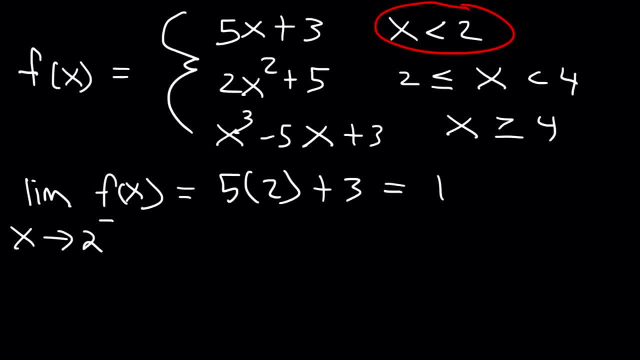 2 plus 3, which is 10 plus 3, so that's equal to 13.. Now what is the limit? as x approaches, 2 from the right of f, of x On the right side, that is greater than 2.. We need to use this portion of the piecewise function: 2x squared plus 5.. So it's 2 times 2 squared plus 5.. 2 squared is 4.. 2 times 4 is 8.. 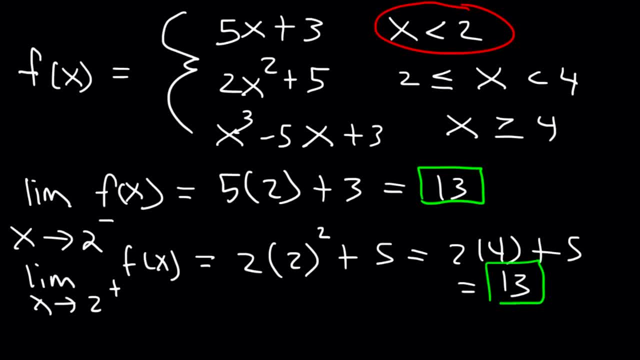 Plus 5 is 13.. Now let's find the limit as x approaches 2 from either side. So because these two are the same, you know that it's going to be 13.. Now here's the next question: What is the value of f of 2?? 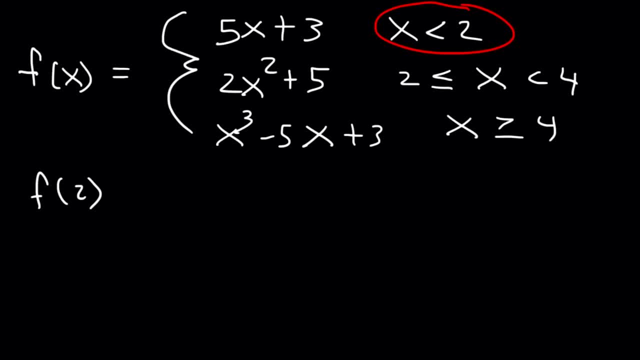 Which function or which portion of the piecewise function should we use to find the value of f of 2?? So x doesn't equal 2 for this particular portion of the function, but it does equal 2 in this function. So we're going to have to use 2x squared plus 5, which we already know what the answer is. 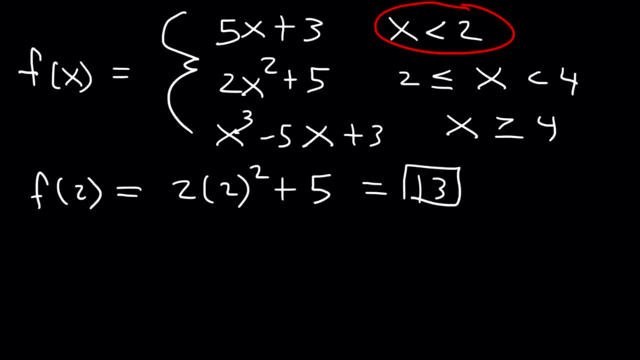 This is equal to 13.. So f of 2 is defined. Now what is the limit As x approaches 4 from the left side? So from the left side of 4, that is, when x is less than 4.. 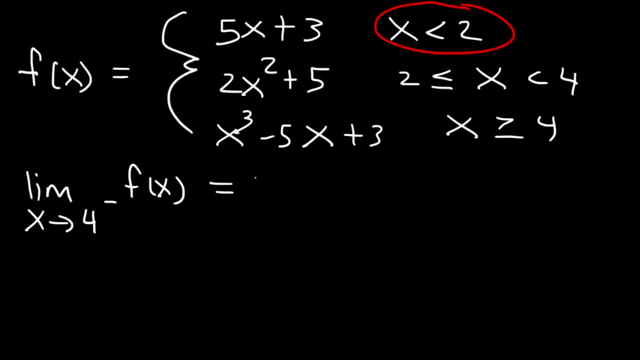 We need to use 2x squared plus 5.. So it's going to be 2 times 4 squared plus 5.. 4 squared is 16.. 2 times 16 is 32.. 32 plus 5, well, that's equal to 37.. 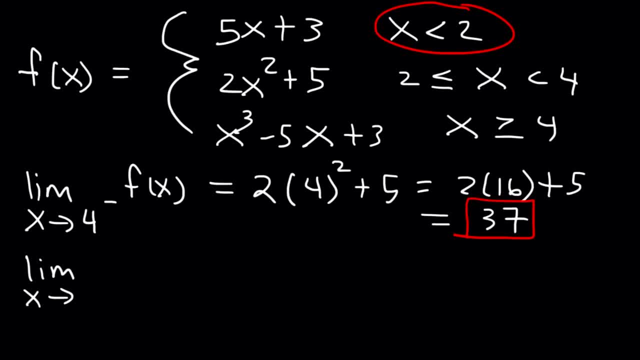 Now what is the value of of the limit as x approaches 4 from the right side? This time x has to be greater than 4.. So we need to use this portion of the piecewise function. So let's plug in 4.. 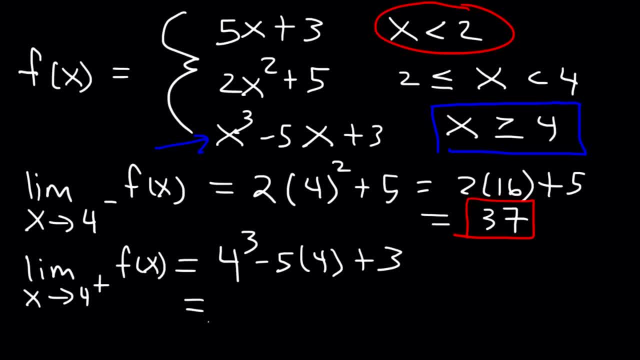 4 to the 3rd. 4 times 4 is 16 times 4, that's 64.. 5 times 4 is 20.. And 64 minus 20 is 42.. And 44 plus 3, that's 47.. 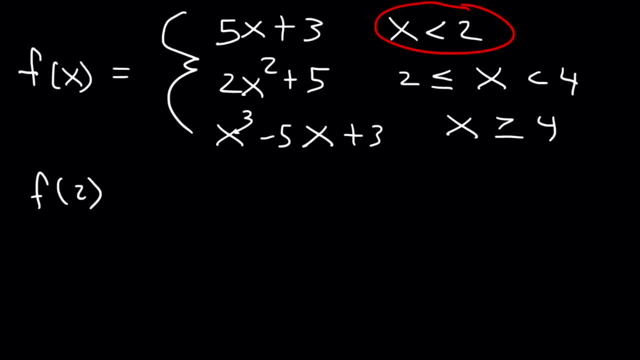 Now here's the next question: What is the value of f of 2?? Which function or which portion of the piecewise function should we use? Let's define the value of f of 2.. So x doesn't equal 2 for this particular portion of the function, but it does equal 2 in this function. 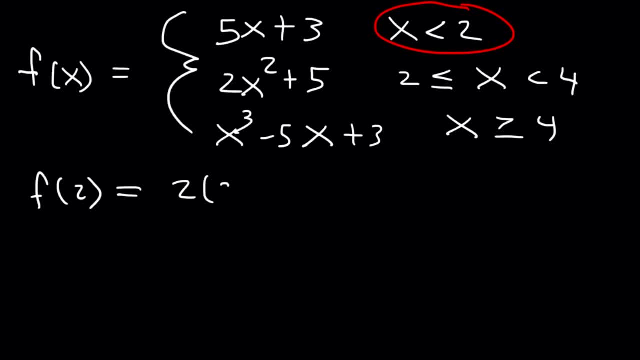 So we're going to have to use 2x squared plus 5, which we already know what the answer is: This is equal to 13.. So f of 2 is defined. Now what is the limit as x approaches 4 from the left side? 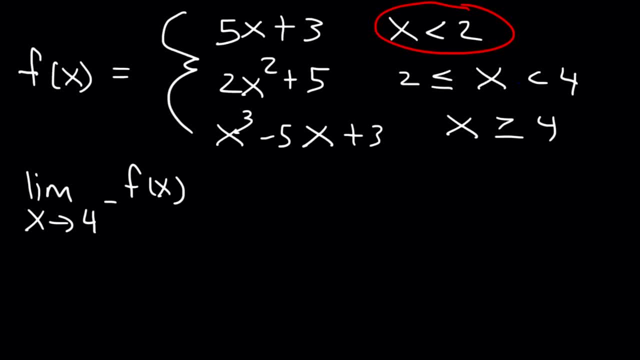 So from the left side of 4, that is, when x is less than 4, we need to use 2x squared plus 5.. So it's going to be 2 times 4 squared plus 5.. 4 squared is 16.. 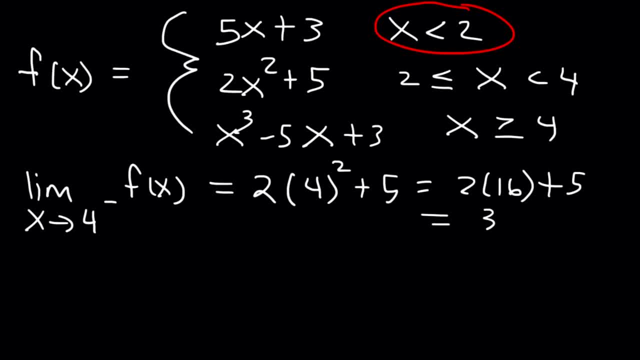 2 times 16 is 32.. 32 plus 5,- well, that's equal to 37.. Now what is the value of the limit as x approaches 4 from the right side. This time x has to be greater than 4.. 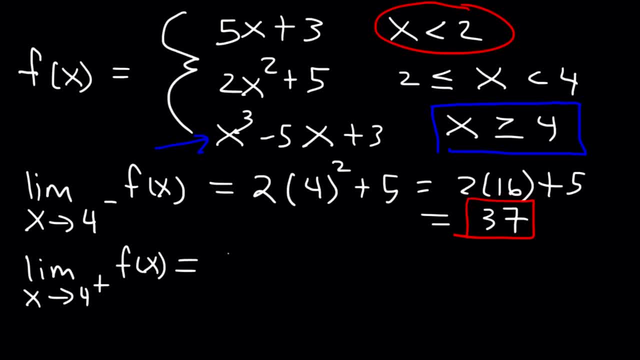 So we need to use this portion of the piecewise function. So let's plug in 4.. 4 to the 3rd: 4 times 4 is 16.. 16 times 4,, that's 64.. 5 times 4 is 20.. 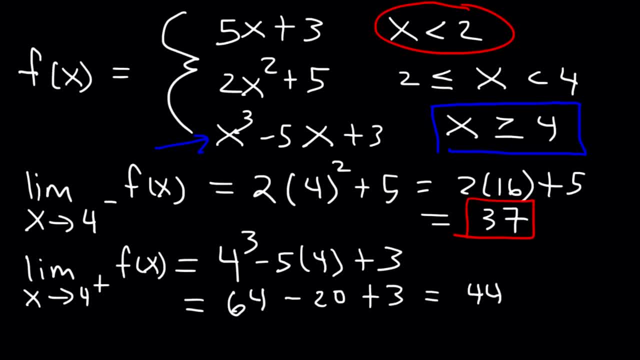 And 64 minus 20 is 44. And 44 plus 3, that's 47. So even though the one-sided limits exist, because they don't match, the limit itself does not exist. So the limit as x approaches 4 from either side does not exist in this particular problem. 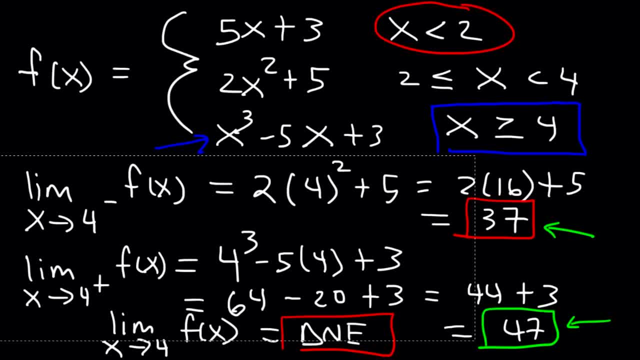 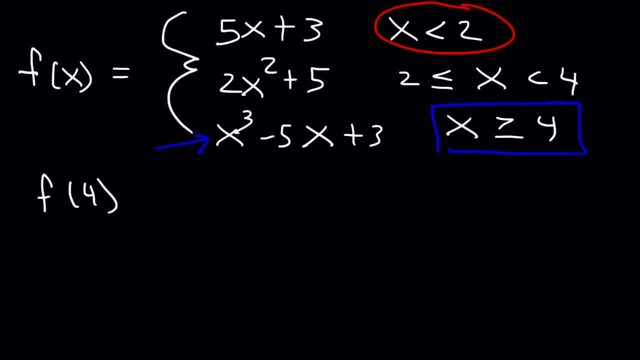 Now there's one more question that we need to answer. What is the value of f of 4?? So when x is 4, what is the value of the function x is 4 using this portion of the piecewise function? 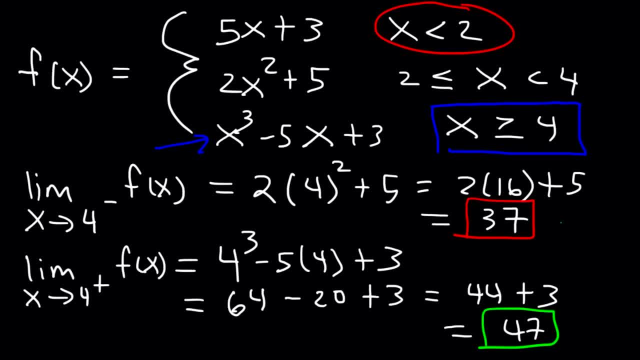 So even though the one-sided limits exist, because they don't match, the limit itself does not exist. So the limit as x approaches 4 from either side does not exist in this particular problem. Now there's one more question that we need to answer. 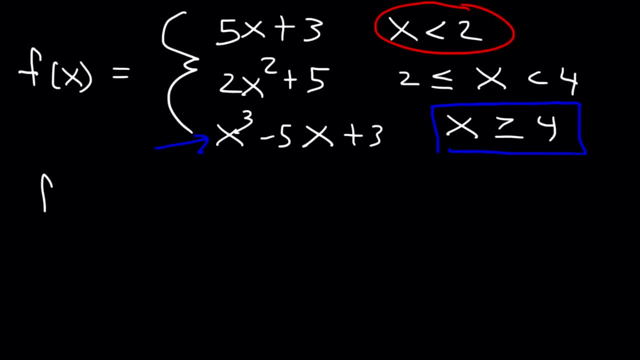 What is the value of f of 4?? So, when x is 4, what is the value of the function? x is 4 used in this portion of the piecewise function, And so, as we mentioned before, this is going to be 47.. 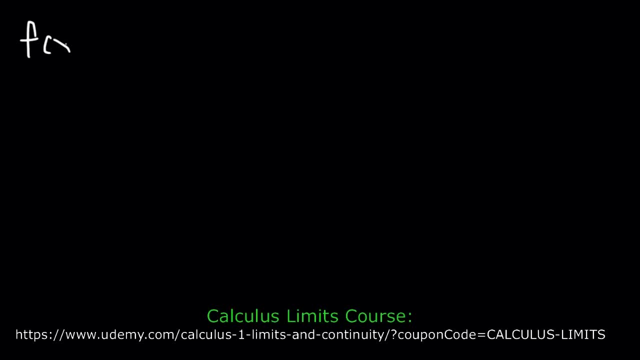 So let's work on another example. So here's another piecewise function. When x is less than 1, we have the portion 7x minus 5. And then the function is going to be equal to 3x squared minus x. 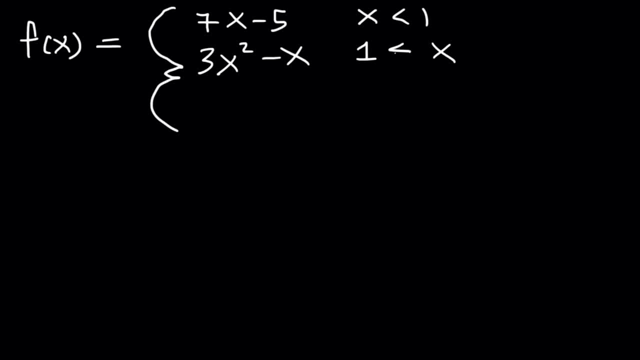 When x is greater than 1, but less than or equal to 3.. Now the function will have a value of 5 when x is equal to 1.. And it's going to be equal to 3.. And it's going to be x cubed plus 4 when x is greater than 3.. 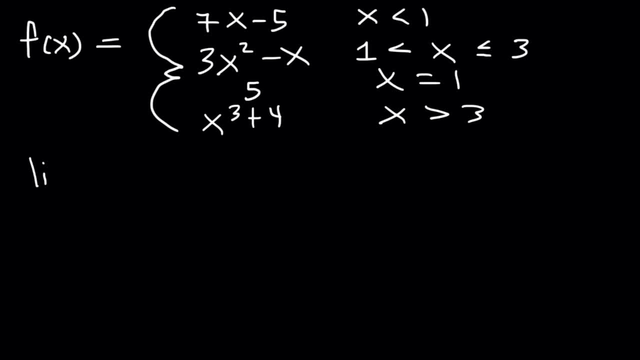 So, using this information, what is the limit? as x approaches positive 1 from the left side, So 1 from the left side, that's less than 1.. So therefore we have to use 7x minus 5.. 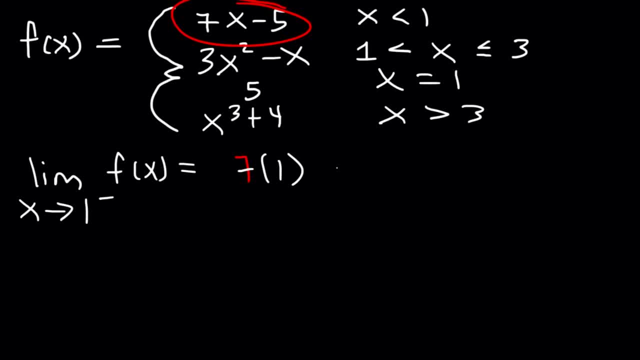 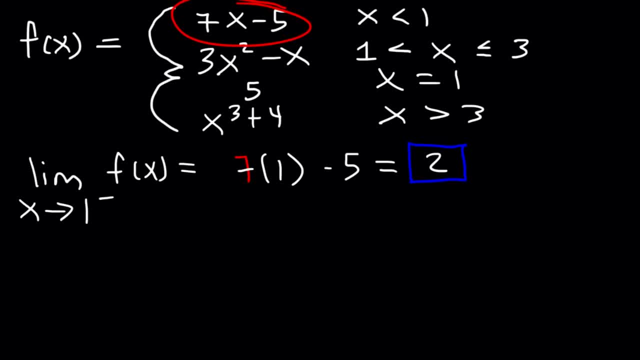 7 minus 5 is 2.. So that's the value of the left-sided limit. Now what about the right-side limit As x approaches 1 from the right side? what is the value of f of x? So this time we need to use 3x squared minus x. 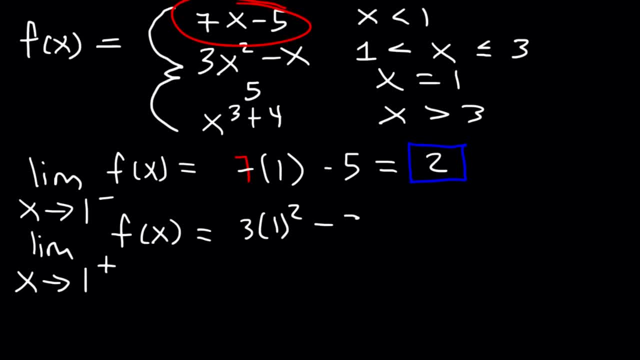 1 squared is 1 times 3.. That's 3 minus 1. That's going to be equal to 2.. So because these two, the left-sided limit and the right-sided limit, because they're the same, the limit as x approaches, 1 from either side will also be equal to 2.. 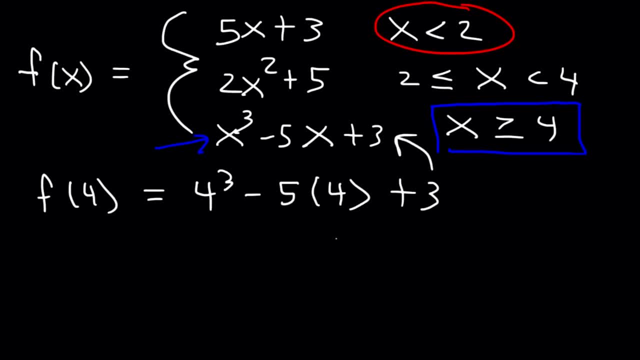 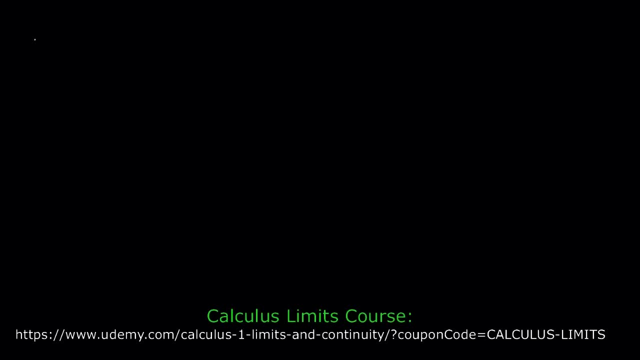 And so, as we mentioned before, this is going to be 47. So let's work on another example. So here's another piecewise function: When x is less than 1, we have the portion 7x minus 5.. 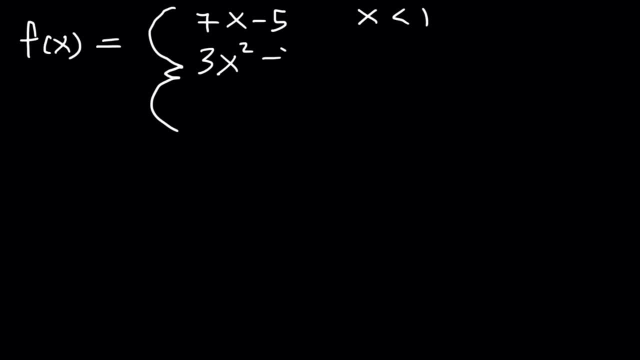 And then the function is going to be equal to 3x squared minus x when x is greater than 1, but less than or equal to 3.. Now the function will have a value of 5 when x is equal to 1.. 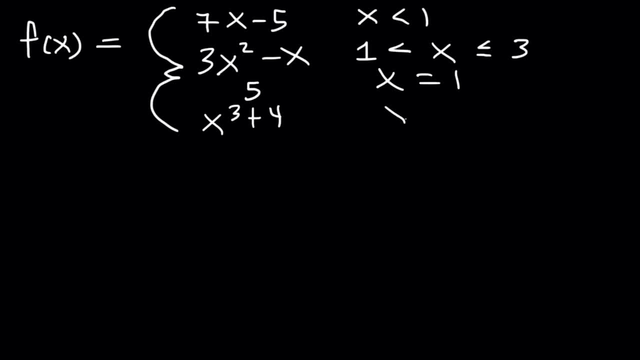 And it's going to be x cubed plus 4, when x is greater than 3.. So, using this equation, we're going to have a value of 5.. using this information, what is the limit as X approaches positive? one from the left side. so one from the left side. that's less than one. so therefore we 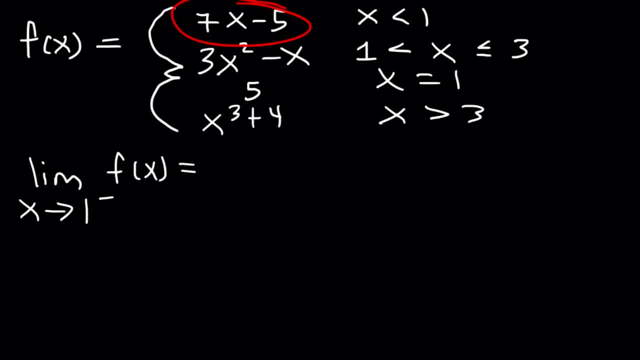 have to use 7x minus 5, so that's going to be 7 times 1 minus 5. 7 minus 5 is 2, so that's the value of the left-sided limit. now what about the right side limit as X approaches one from the right side? what is the value of f, of X? so this: 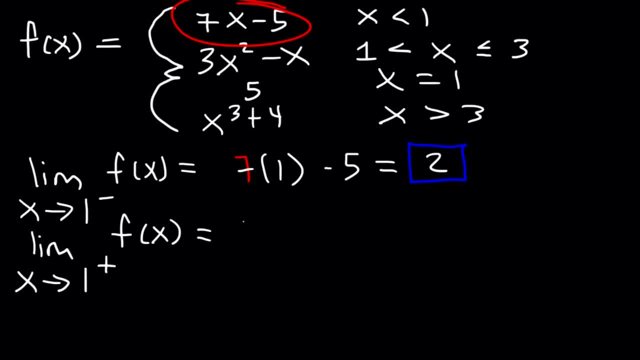 time we need to use 3x squared minus X 1 squared is 1 times 3, that's 3 minus 1. that's going to be equal to 2. so because these two, the left side the limit and the right side limit, because 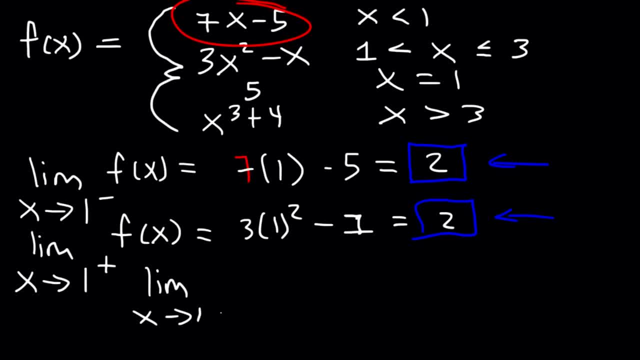 they're the same. the limit as X approaches, one from either side will also be equal to 2. now what is the value of f, of 1? so when X is exactly 1, what is the value of the function? so when X is 1, notice that the value the function is 5. so 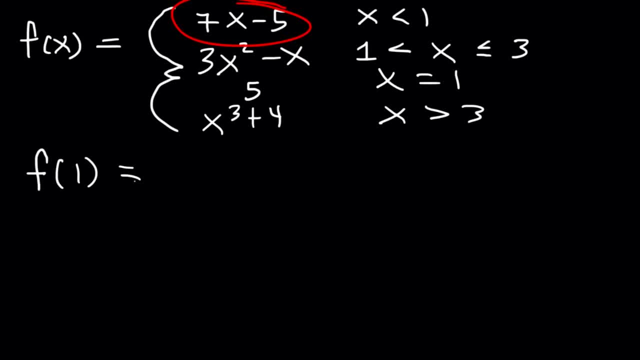 Now, what is the value of f of 1?? So when x is exactly 1,, what is the value of the function? So, when x is 1, notice that the value of the function is 5.. So f of 1 is equal to 5.. 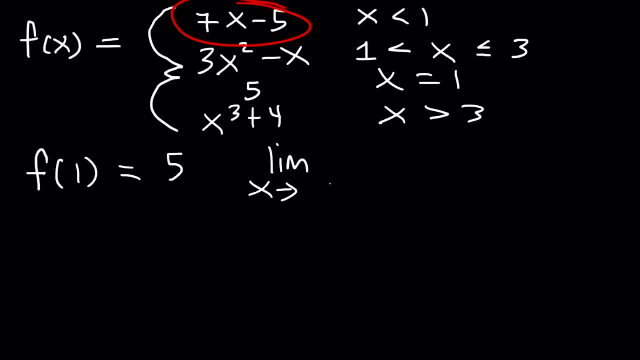 Now what is the limit as x approaches 3 from the left side, So that's when x is less than 3.. So we got to use 3x squared minus x, So let's plug in 3.. It's going to be 3 times 3 squared minus 3.. 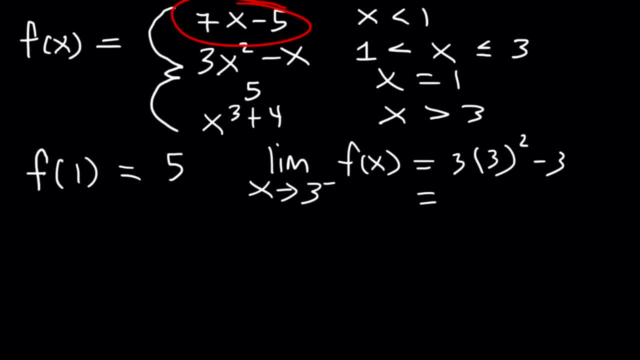 3 squared is 9 times 3.. That's 27.. 27 minus 3 is 24.. Now what about the right-sided limit? What is the limit as x approaches 3 from the right side? So when x is greater than 3, we need to use this portion of the equation. 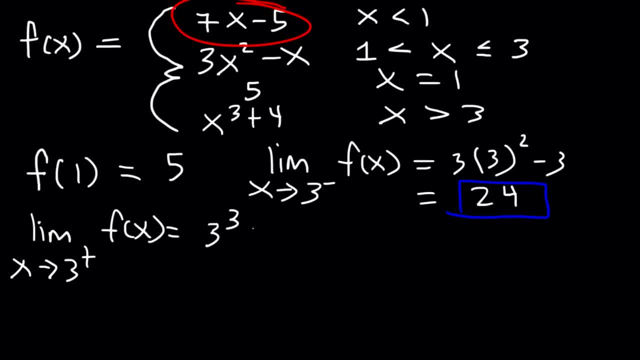 So x cubed plus 4.. So it's going to be 3 to the 3rd plus 4.. That's 27 plus 4, which is 31.. So that's the limit. as x approaches 3 from the right side. 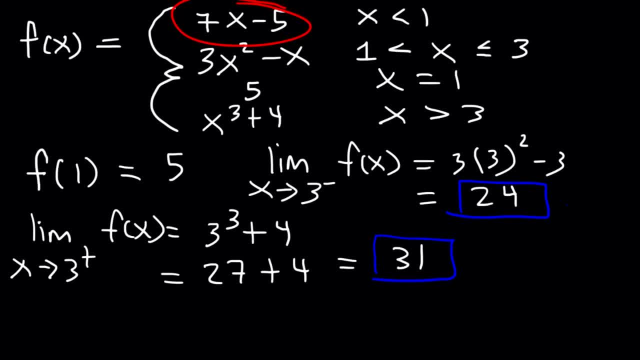 So the left-sided limit and the right-sided limit. there's a mismatch, They don't equal the same thing. Therefore, the limit as x approaches 3 from either side, we could say, does not exist. Now what is the value of f of 3?? 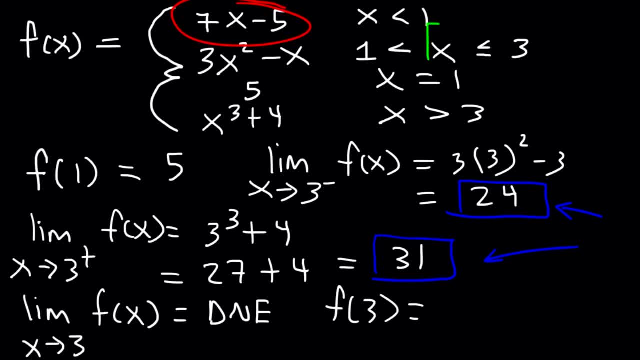 To find the value of f of 3, we need to use this portion, because x is less than and equal to 3.. When we plug in 3 into 3x, squared minus x, we got 24.. So f of 3 is 24.. 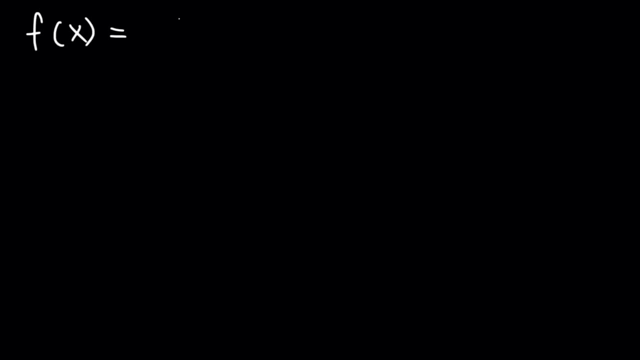 Consider the function f of x, which is equal to cx plus 3 when x is less than 2.. And that's equal to 3x plus c when x is equal to or greater than 2.. What is the value of the constant c that will make the function continuous at x equals 2?? 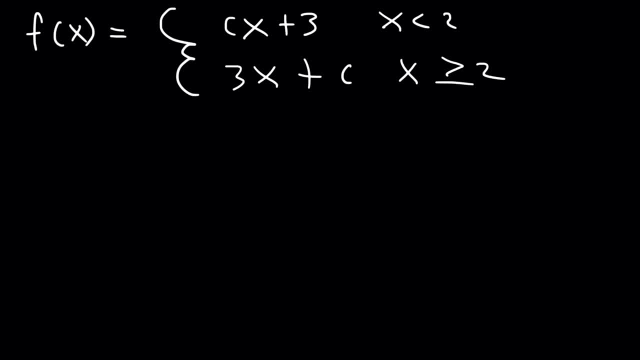 So what do we need to do in order to find the value of that constant c? Well, if it's going to be continuous, at x equals 2,, these two functions have to have the same y value, which means that they must be equal to each other. 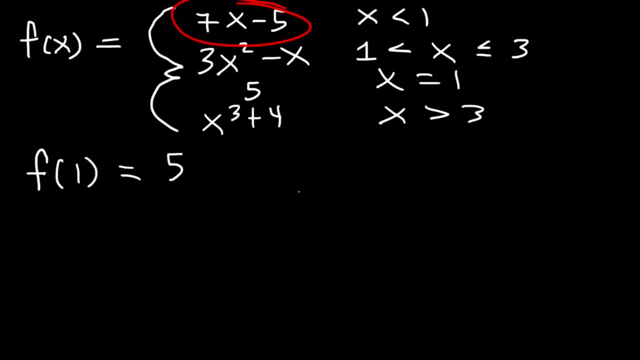 f of one is equal to 5. now what is the limit as X approaches stree from the left side. so that's wheln, X is less than 3. so we gotta use 3x squared minus X. so let's plug in three, three times three squared minus 3. 3 squared is 9 times 3, dance 2727. 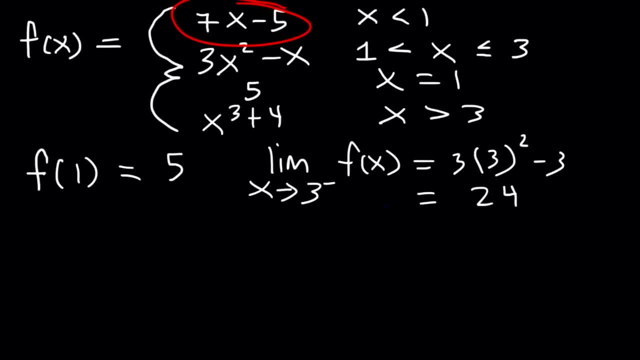 minus 3 is 24. 3 squared is 9 times 3, that's 27. 27 minus 3 is 24. Now what about the right-sided limit? What is the limit as X approaches 3 from the right side? So when X is greater than 3, we need to use this portion of the equation. 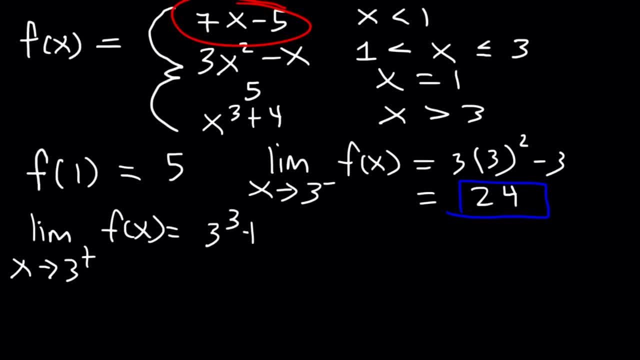 So X cubed plus 4.. So it's going to be 3 to the third plus 4.. That's 27 plus 4, which is 31.. So the left-sided limit and the right-sided limit. there's a mismatch. 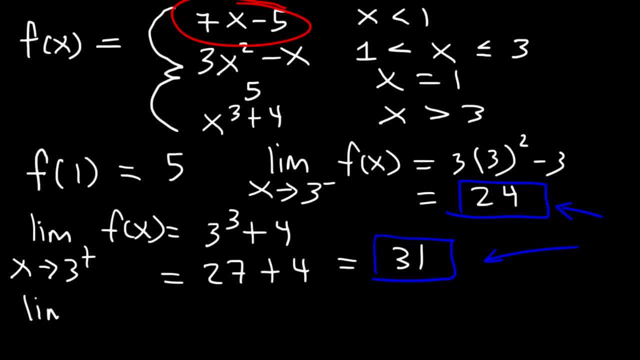 They don't equal the same thing. Therefore, the limit as X approaches 3 from either side we could say- does not exist. Now what is the value of F of 3?? To find the value of F of 3, we need to use this portion, because X is less than and equal. 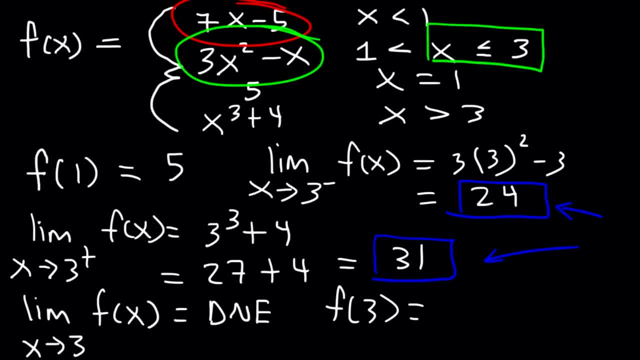 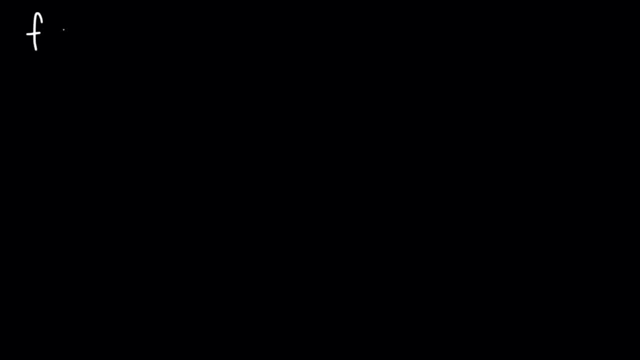 to 3.. When we plug in 3 into 3X squared minus X, we got 24.. So F of 3. It's 24.. Consider the function F of X, which is equal to CX plus 3 when X is less than 2.. 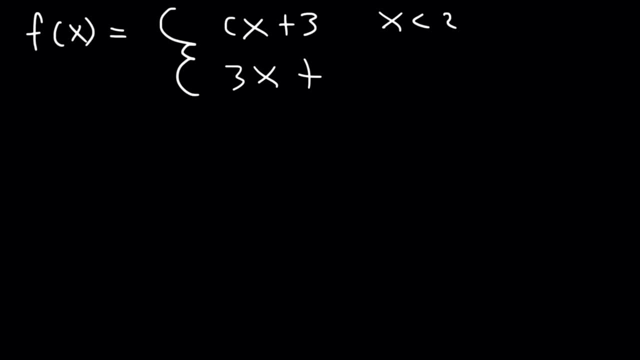 And that's equal to 3X plus C when X is equal to or greater than 2.. What is the value of the constant C that will make the function continuous at X equals 2?? Well, we're going to look at this function again. 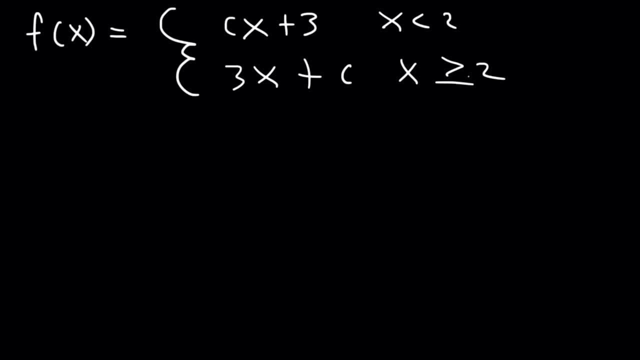 This function will not be continuous in any time. It will still end at X final. It's still going to leave a constant area. j donc tu se summone et on tour, je suis un느�au At that. personal from the next column leave a constant area. 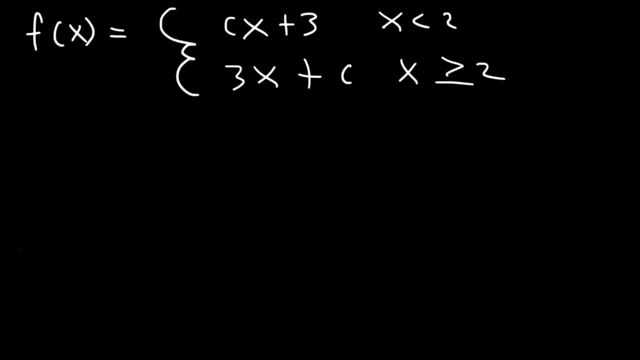 So what do we need to do in order to find the value of that constant C? Well, if it's going to be continuous, at X equals 2,, these two functions have to have the same Y value, which means that they must be equal to each other.